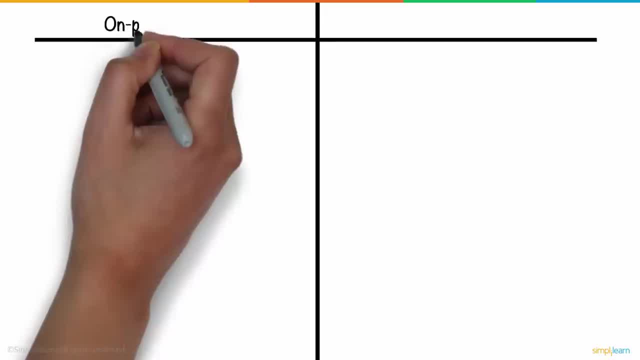 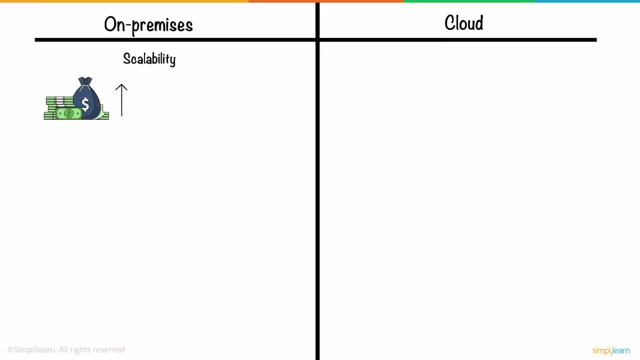 investing money into it. you decide to draw up the differences between on-premise and cloud-based computing to make a better decision When it comes to scalability. you pay more for an on-premise setup and get lesser options too. Once you've scaled up, it is difficult. 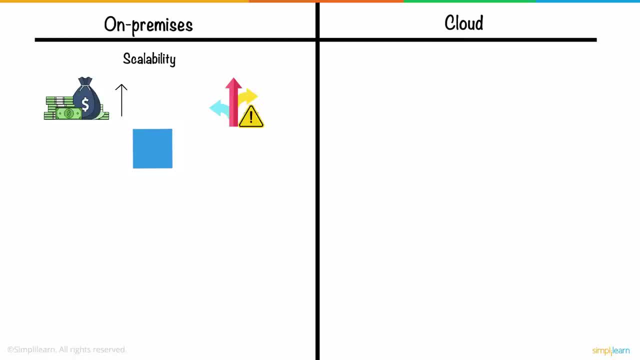 to scale down and often leads to heavy losses in terms of infrastructure and maintenance costs. Cloud computing, on the other hand, allows you to pay only for how much you use, with much easier and faster provisions for scaling up or down. Next, let's talk about server storage. On-premise systems need a lot of space for their servers. 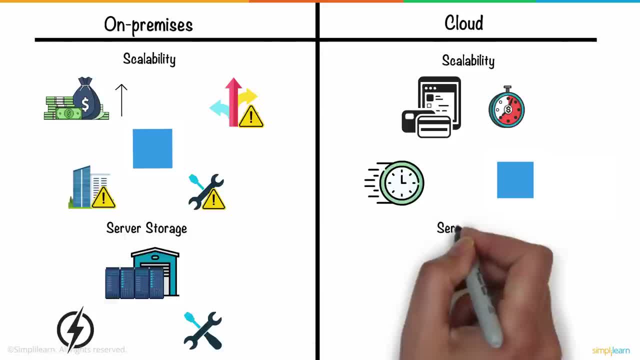 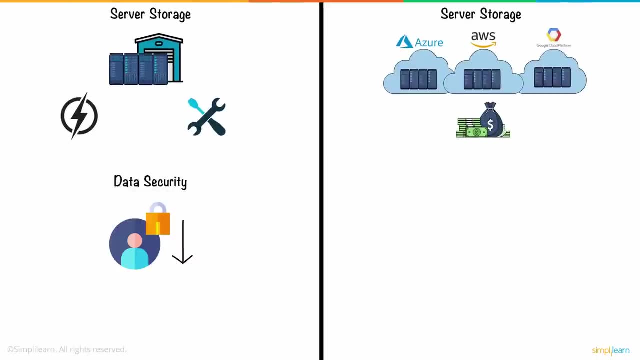 notwithstanding the power and maintenance hassles that come with them. On the other hand, cloud computing solutions are offered by cloud service providers who manage and maintain the servers, saving you both money and space. Then we have data security. On-premise systems offer less data security thanks to a complicated 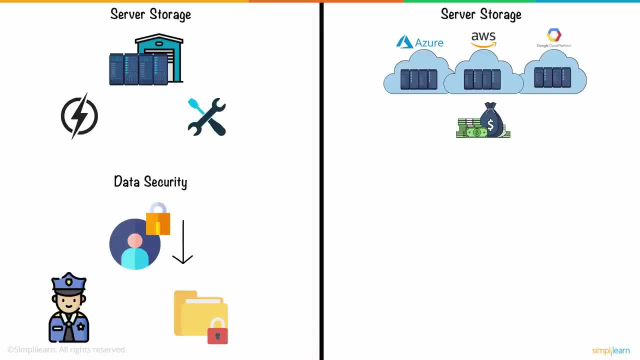 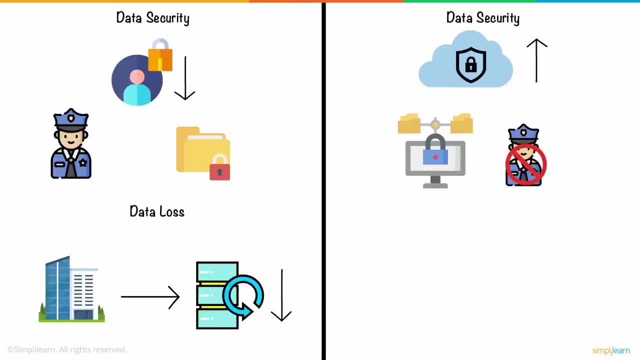 combination of physical and traditional IT security measures, whereas cloud computing systems offer much better security and let you avoid having to constantly monitor and manage security protocols. In the event that a data loss does occur, the chance for data recovery with on-premise setups are very small. In contrast, 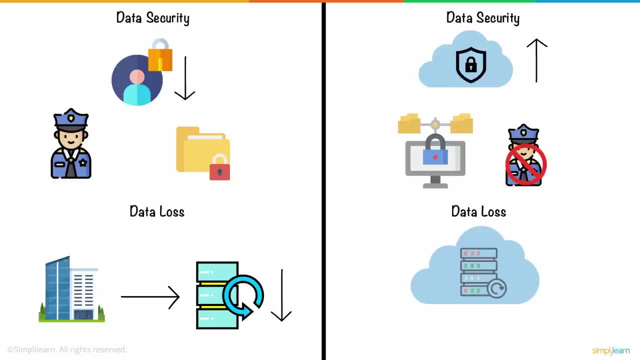 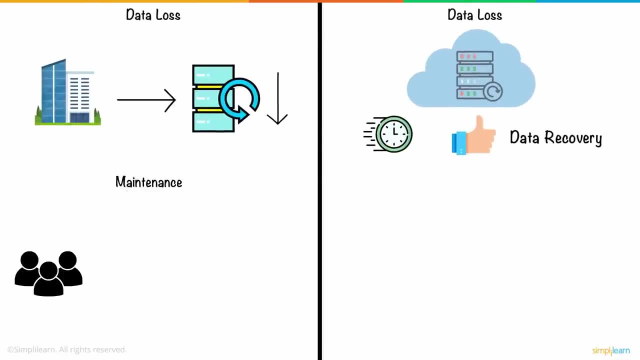 cloud computing systems have robust disaster recovery measures in place to ensure faster and easier data recovery. Finally, we have maintenance. On-premises systems also require additional teams for hardware and software maintenance, loading up the costs by a considerable degree. Cloud computing systems, on the other hand, are maintained by the cloud service providers. 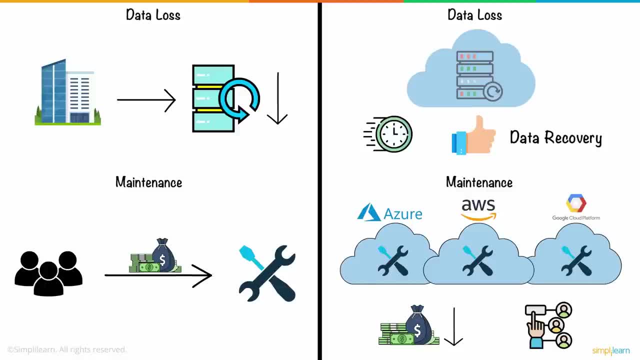 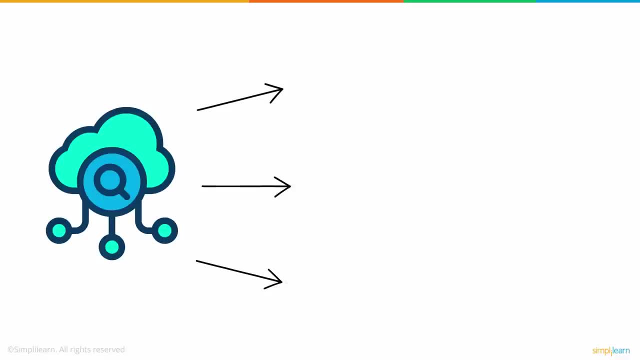 reducing your costs and, in turn, reducing your resources and making your resources more efficient. So if you're thinking about cloud computing as an option, you should take a closer look at what exactly cloud computing is. Cloud computing refers to the delivery of on-demand computing services over the internet on a pay-as-you-go basis. 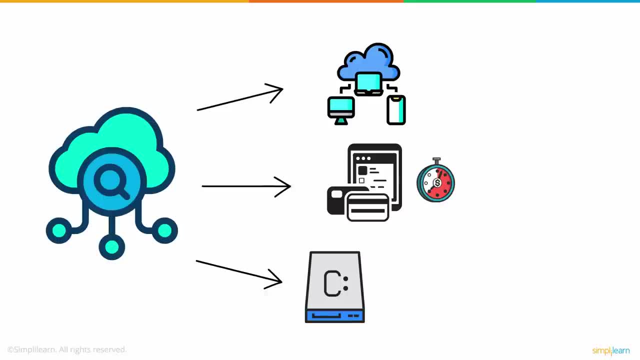 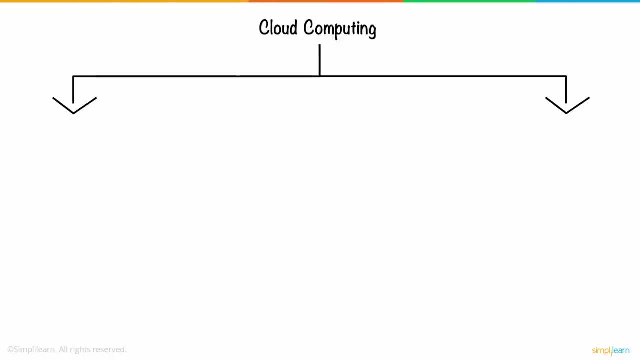 In simpler words, rather than managing files and services on a local storage device, you'll be doing the same over the internet in a cost-efficient manner. Cloud computing has two types of models — deployment model and service model. There are three types of deployment models – public, private and hybrid cloud. 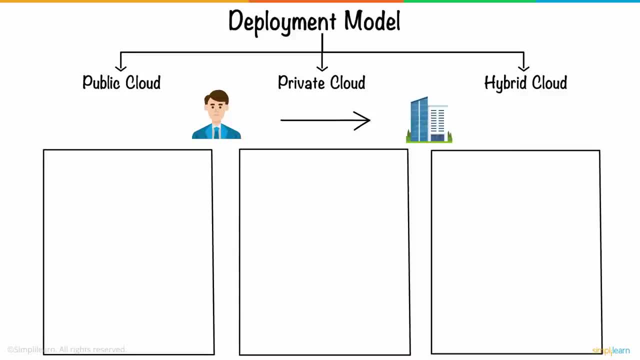 Imagine you're traveling to work. You've got three options to choose from. One you have buses, which represent public clouds. In this case, the cloud infrastructure is available to the public over the internet. These are owned by cloud service providers. 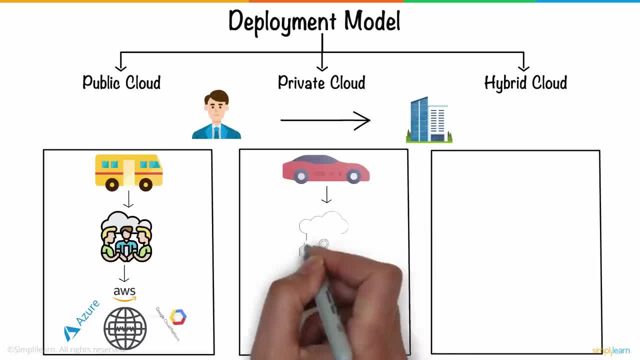 Two. then you have the option of using your own car. This represents the private cloud. With the private cloud, the cloud infrastructure is exclusively operated by a single organization. This can be managed by the organization or a third party. And finally, you have the option to hail a cab. 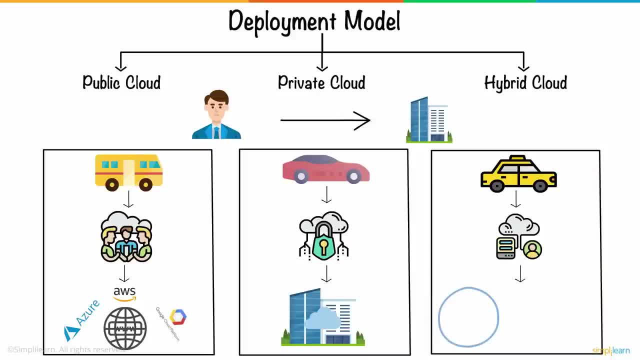 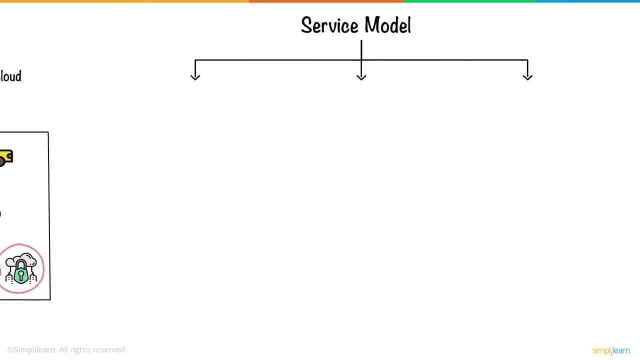 This represents the hybrid cloud. A hybrid cloud is a combination of the functionalities of both public and private clouds. Next, let's have a look at the service models. There are three major service models available – EAS, PAS and SAS. Compared to on-premises. 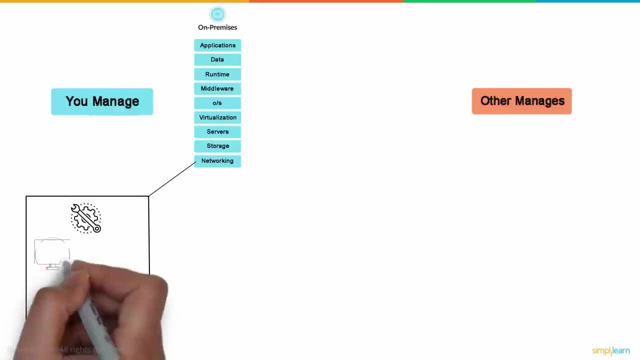 where you'll need to manage and maintain every component – including applications, data, virtualization and middleware – cloud computing service models are hassle-free. EAS refers to infrastructure as a service. It is a cloud service model where users get access to basic computing infrastructure. 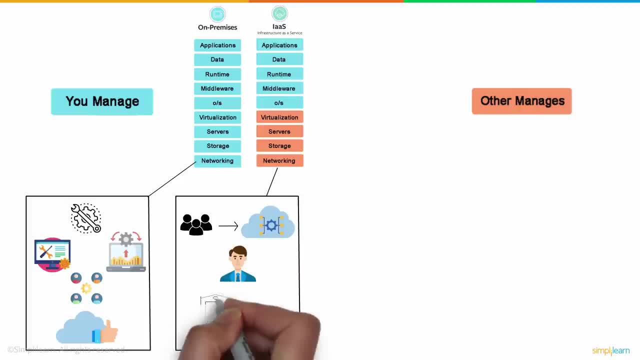 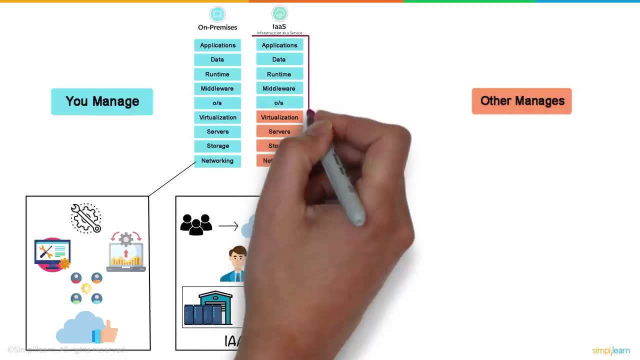 They are commonly used by IT administrators. If your organization requires resources like storage or virtual machines, EAS is the model for you. You'll only have to manage the data runtime, middleware applications and the OS, while the rest is handled by the cloud providers. 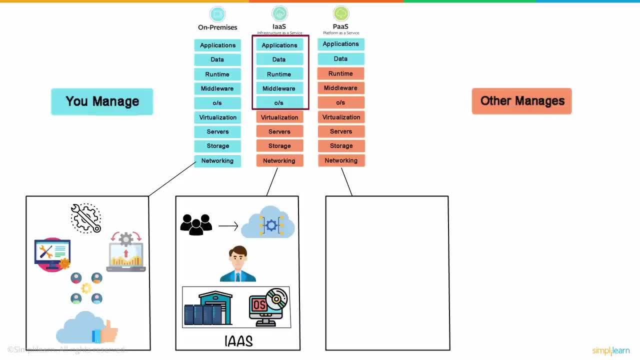 Next we have PAS. PAS or Platform as a Service provides cloud platforms and runtime environments for developing, testing and managing applications. This service model enables users to deploy applications without the need to acquire, manage and maintain the related architecture. 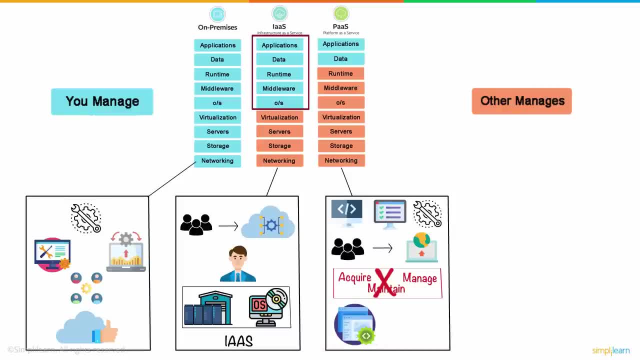 If your organization is in need of a platform for creating software applications, PAS is the model for you. PAS only requires a software application. PAS only requires a software application. PAS only requires a software application. PAS only requires you to handle the applications and the data. 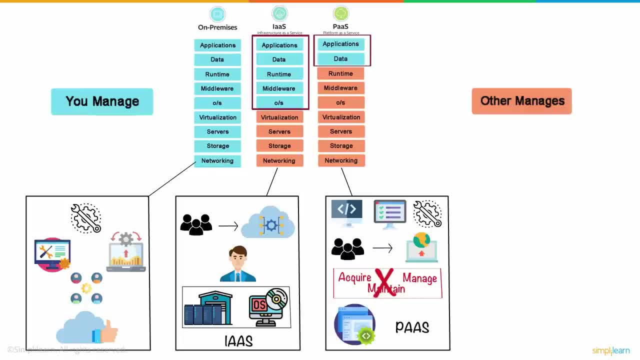 The rest of the components, like runtime, middleware, operating systems, servers, storage and others, are handled by the cloud service providers. And finally, we have SAS. SAS, or Software as a Service, involves cloud services for hosting and managing your software applications.